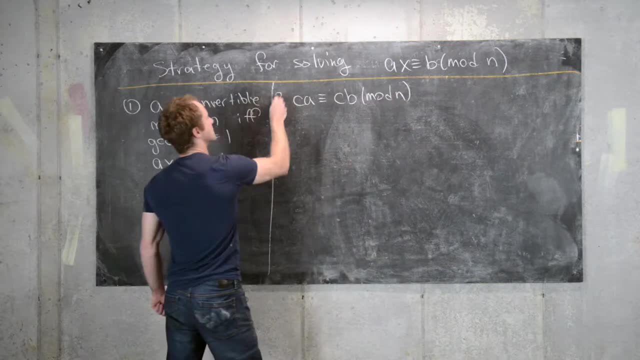 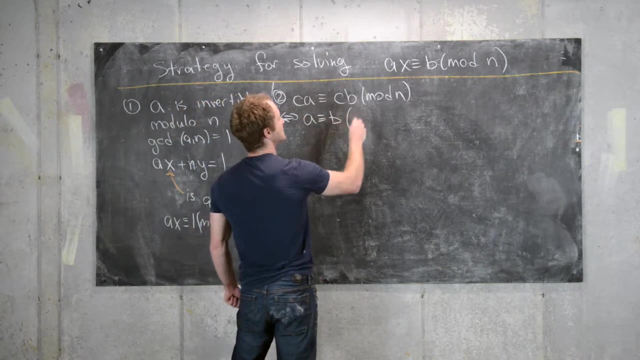 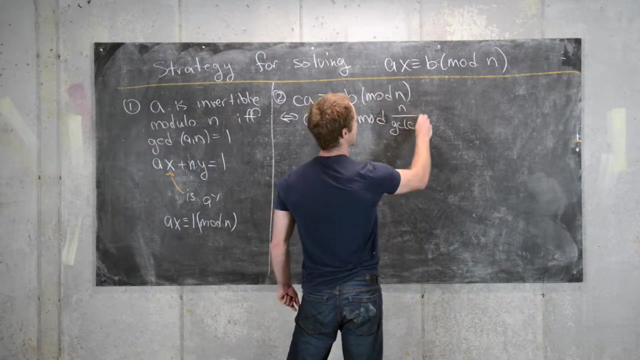 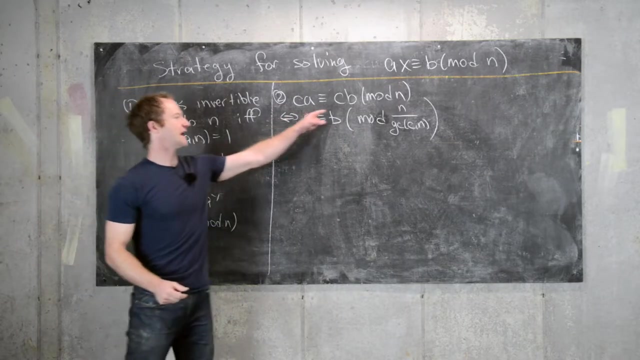 mod N. this is equivalent to saying that A is congruent to B mod N divided by the GCD of C and N. Okay, good, So in other words, you can cancel the C, but you don't land in the same. 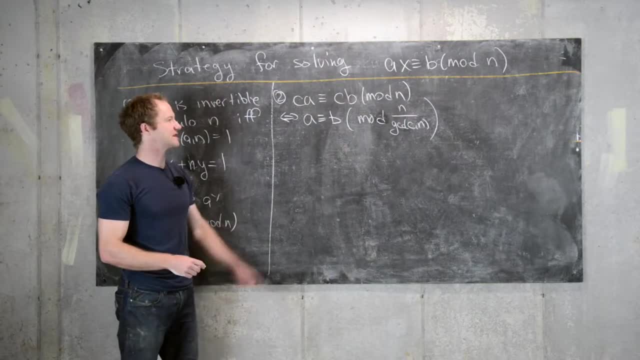 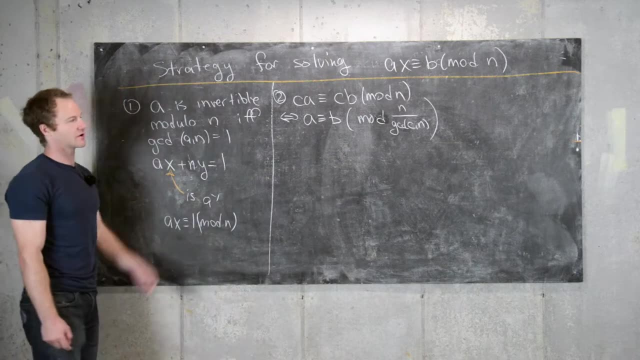 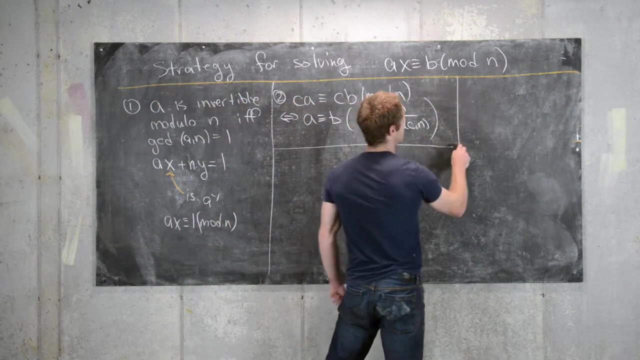 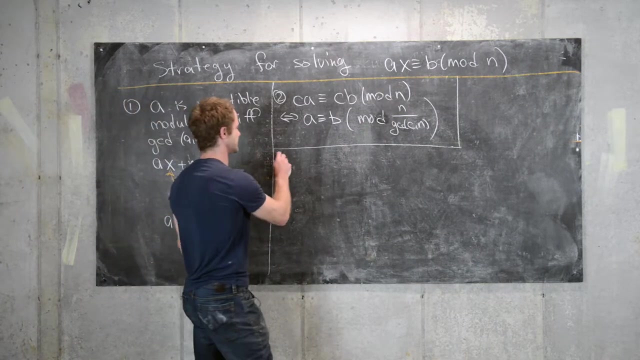 modular space, right? So obviously, if N equals 1, you do land in the same modular space, And that has to do with something over here, but otherwise you don't. Good, So this is one result that's important, Okay, good. So the next one is the following: So number: 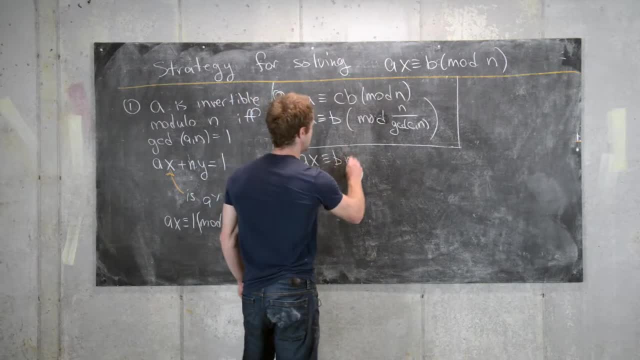 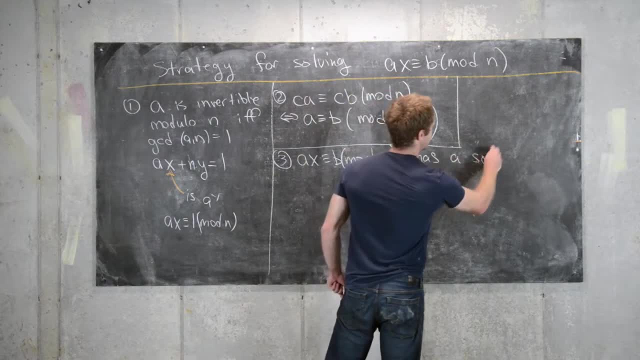 to C mod NY, and this is equivalent to C R mod NY, and this is equivalent to C. Next up is the next example. So we have- I just don't remember right now, but negative function of gender buy. Okay, it's 10 and 10.. That's not rewarded as much, but it feels like. 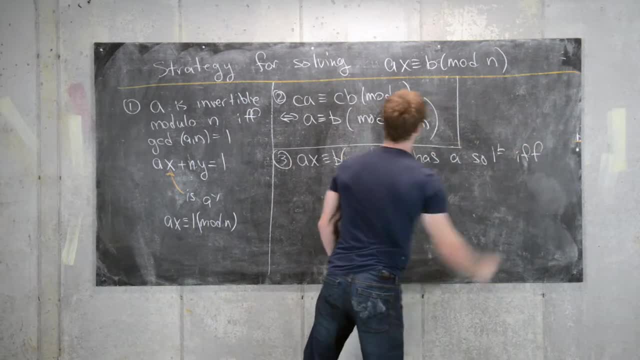 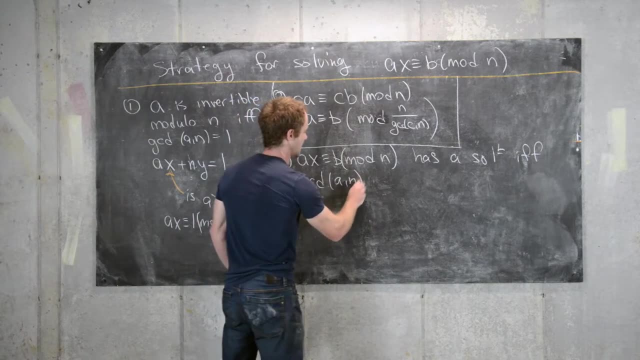 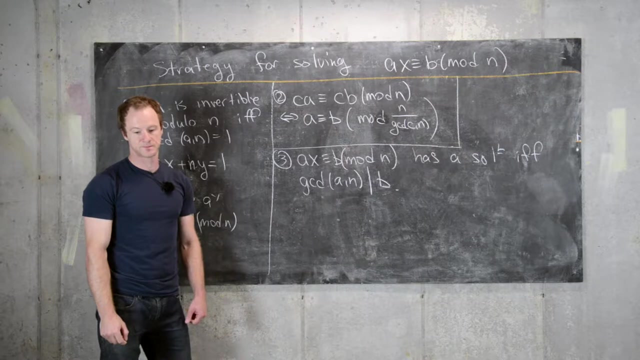 0,, 100 and nothing else, whatever. But at 30, come back. Yeah, TH sided mod equal has to point to C. Two words come to mind: Oh, yeah, good, So the $ 13 have appeared, and then think of the $12 have gone outside, and then thought of the. 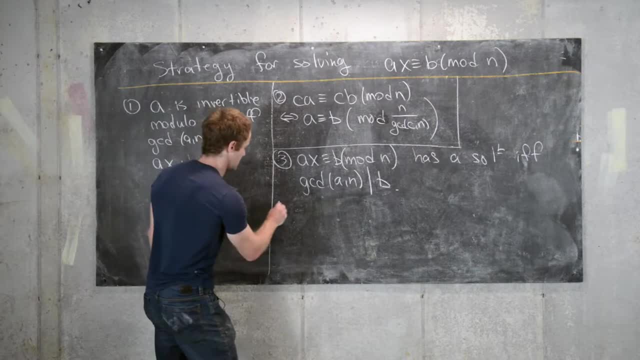 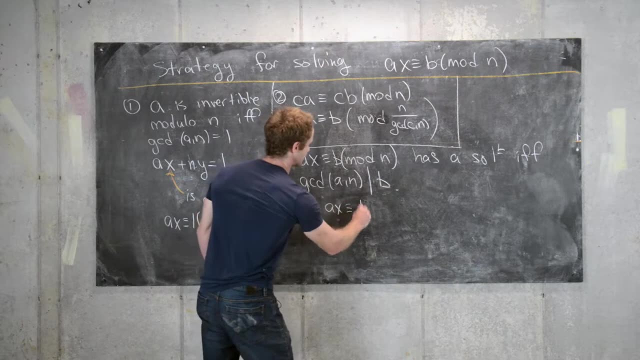 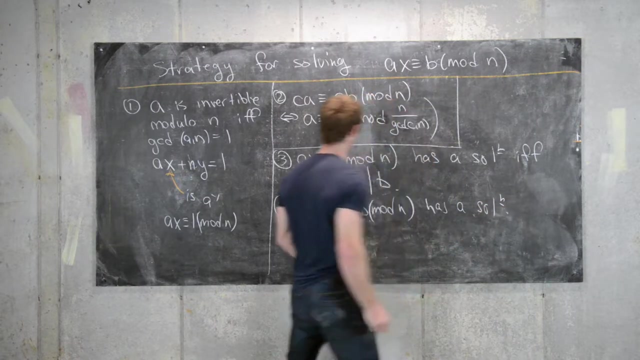 $20 have gone to Club the round. object: $100 have left the middle. what $1, $2,? $1 has left the $2, Because if AX is congruent to B, mod N has a solution. in other words, if the GCD of AN divides B. 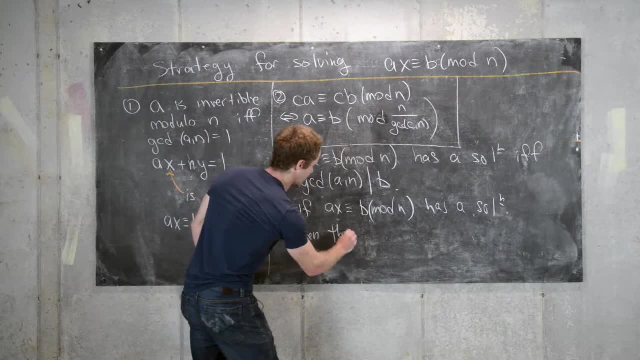 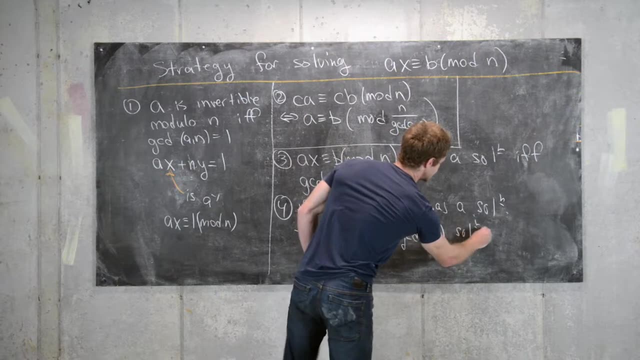 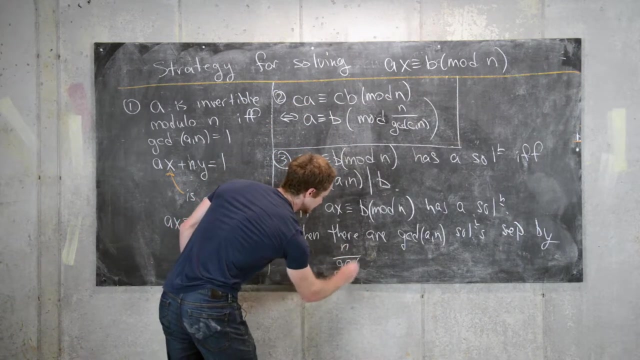 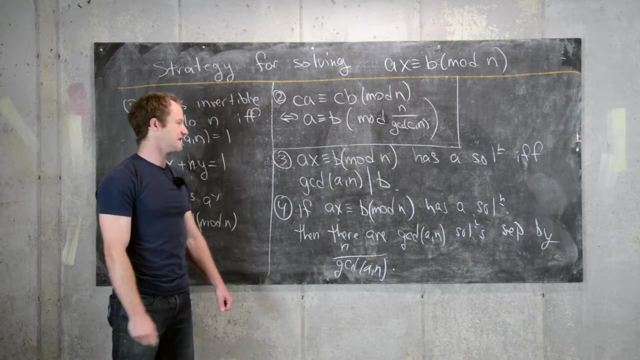 then there are GCD of AN, solutions separated by N, over the GCD of A and N. Okay, good, So now let's clean up the board and we'll look at an example of a couple of these strategies in play. Okay, so we'll look at the following. 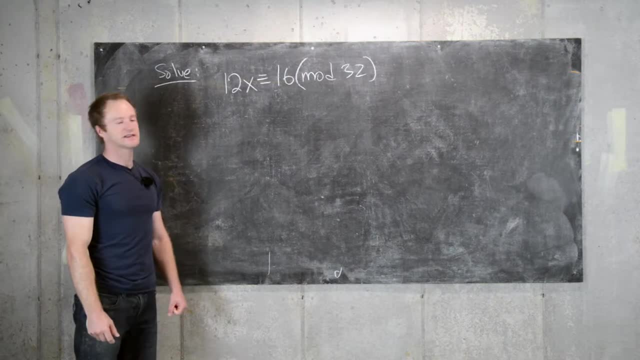 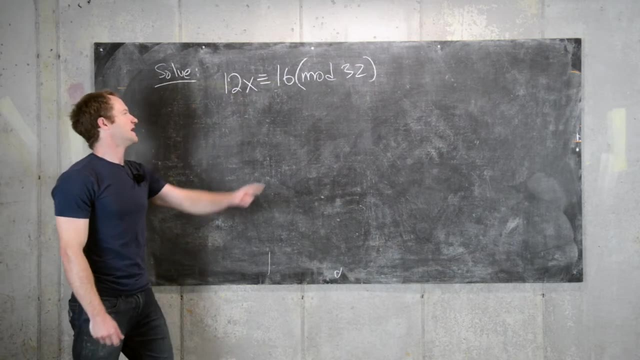 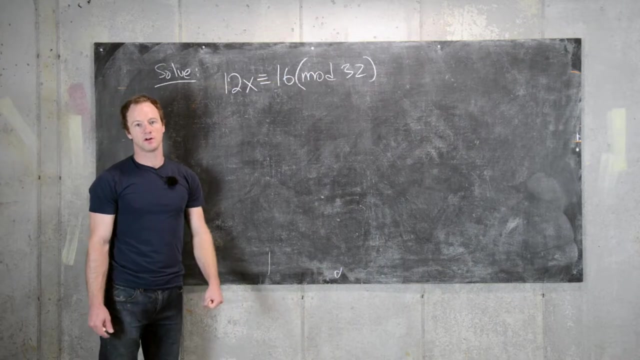 We'll look at the following: linear congruence. So 12X is congruent to 16 mod 32.. So we'll talk through the strategies that were previously on the board. So 12 is not relatively prime to 32.. In other words their GCD is not 1, so we can't just find a multiplicative inverse of 12.. 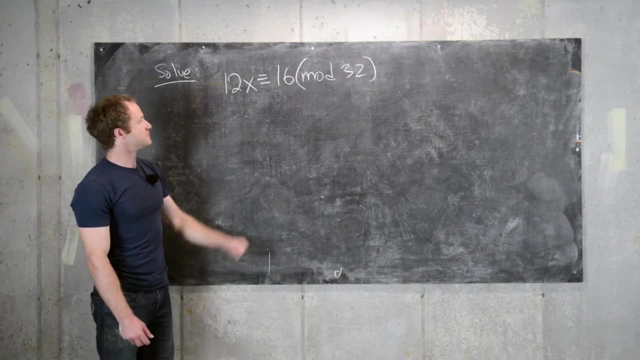 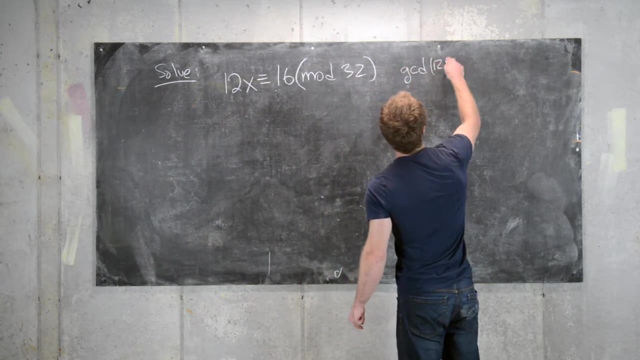 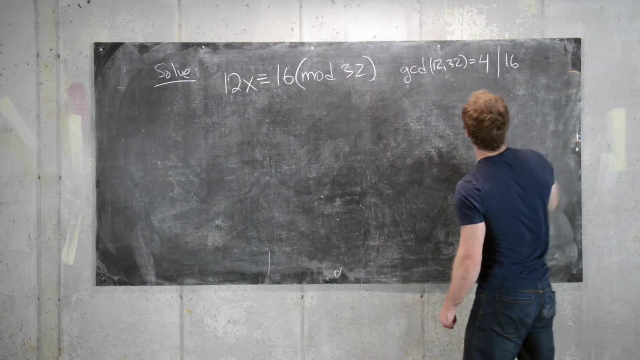 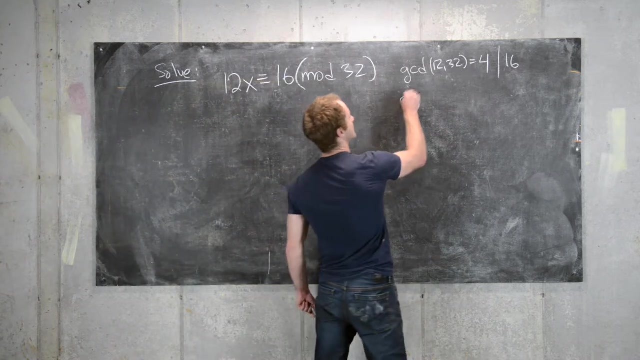 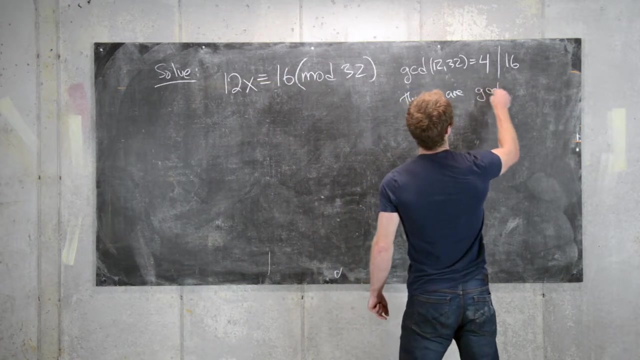 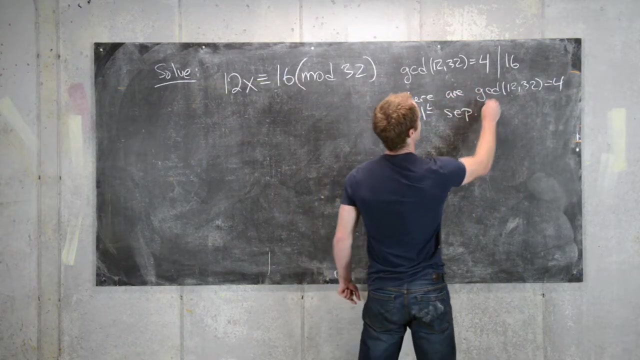 Good, But we see that the GCD of 12.. 12 and 32 equals 4, and 4 divides 16, so there is a solution. Good, So that means we can continue. There is a solution. And furthermore, there are GCD of 12 and 32, so there are 4 solutions separated by. 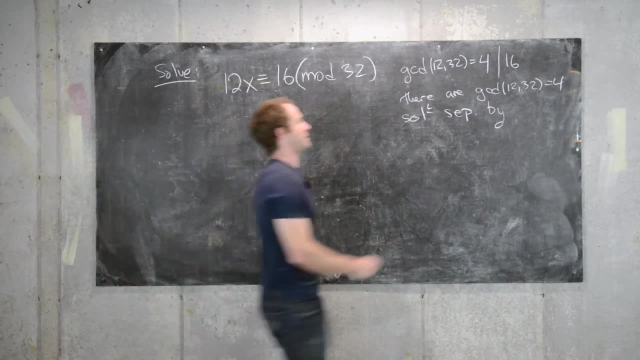 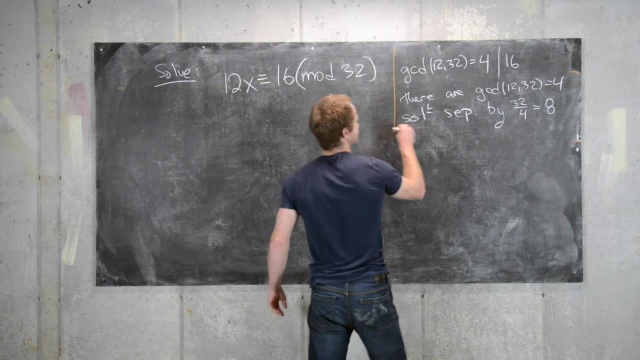 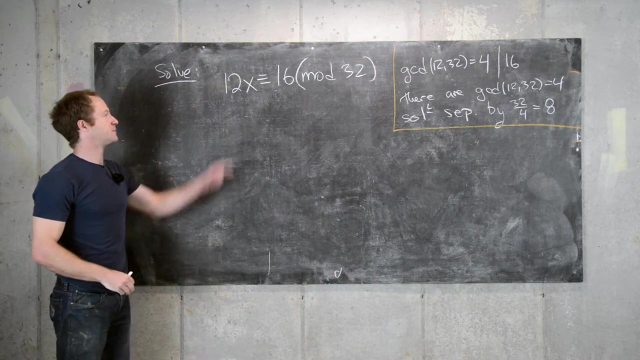 32 divided by 4, which equals 8.. Okay, fantastic. So we boiled it down to the fact that there are 4 solutions, each separated by 8.. So now finding the first solution, we'll use some tricks that were on the previous board. 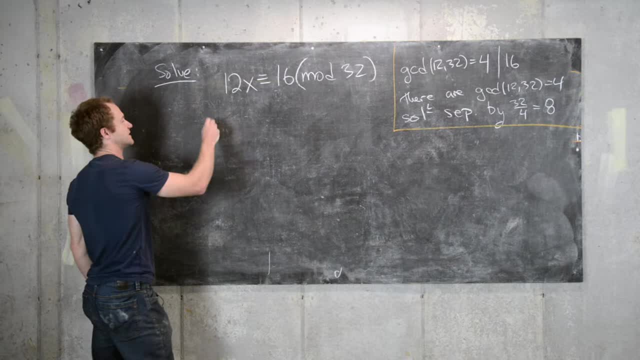 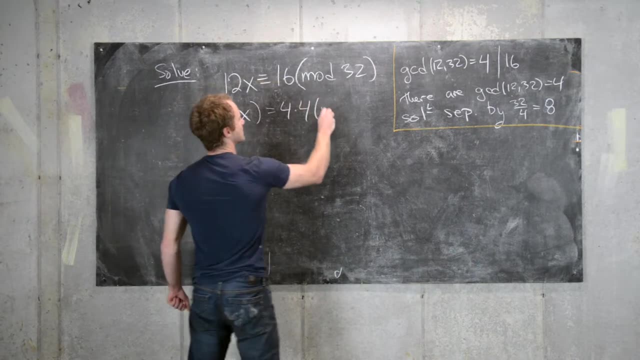 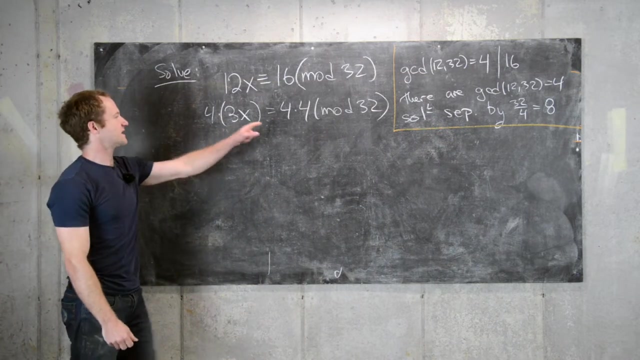 So what we want to first do is maybe factor this out. We can write this as: 4 times 3N. 3X equals 4 times 4,, mod 32.. Okay, good, And this is really good, because this allows us to decrease the number that we're working. 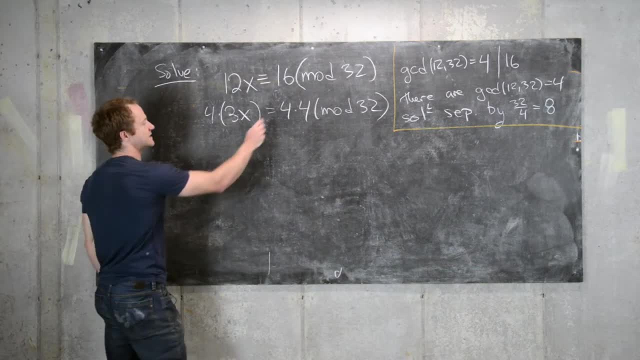 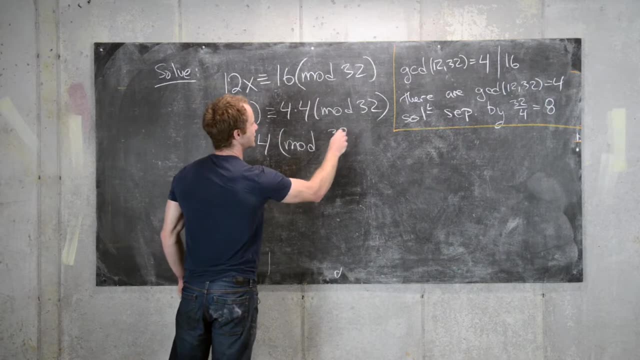 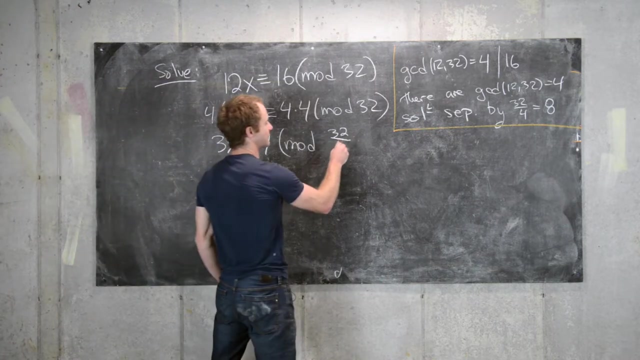 modular with respect to. So this means that 3X is congruent to 4, mod 32, divided by the GCD of 32 and 4, which is 4.. So that is congruent to 4, mod 8.. 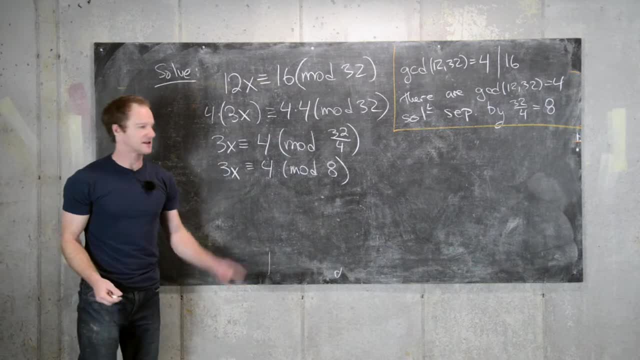 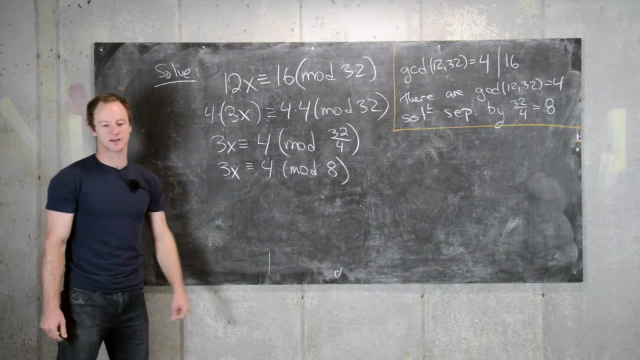 So we have: 3X is congruent to 4, mod 8.. That's equivalent to this. Well, that's not equivalent to this, but if we solve this, then we have solved this linear congruence. Okay, good. 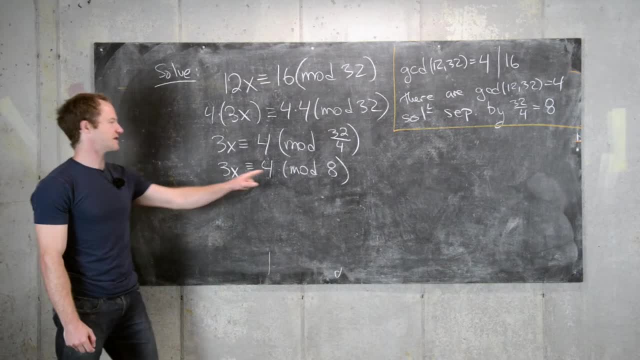 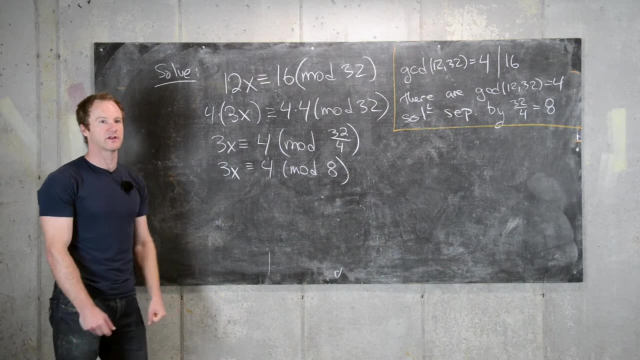 Now what we notice is that 3 is relatively prime to 8, so that means 3 has an inverse modulo 8.. Okay, Now we can use the extended Euclidean algorithm to find this inverse, but since 8 is pretty small, we can guess and check.